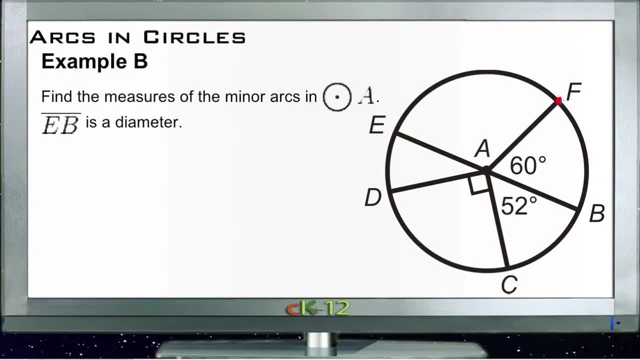 So our first minor arc we'll start right here. We'll start from F and go to B, and that's our first minor arc right down through here, So that one obviously is 60 degrees, We can see that one. So we have arc FB, That one's 60 degrees, And then we have from B. 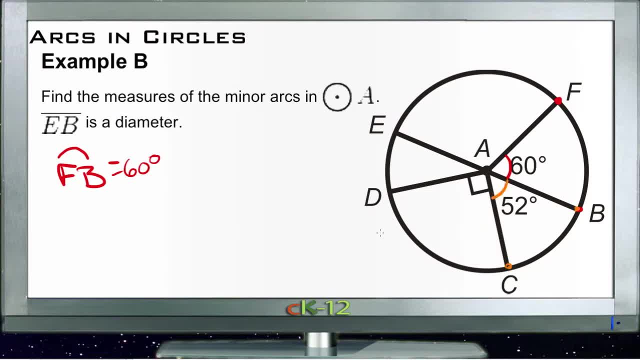 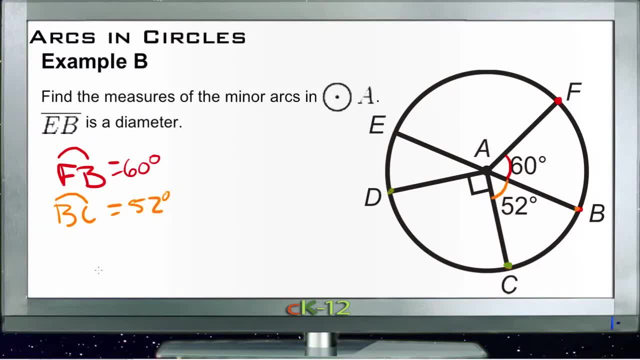 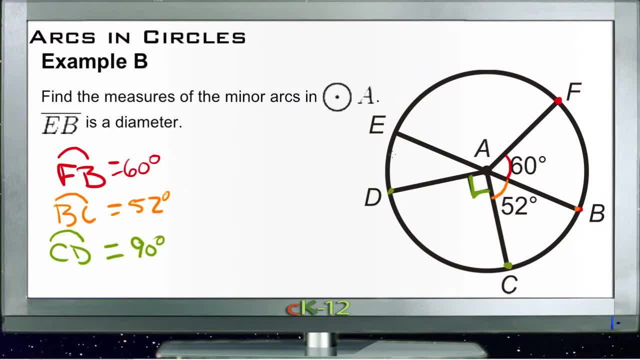 So we know that one's 90 degrees. Now we have DE. DE doesn't have a measure for us here. We're gonna have to calculate that a little bit to get that one. We know that from B all the way around to E is a semicircle, right? 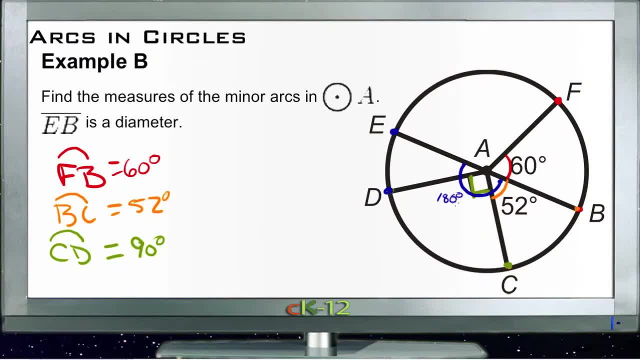 Because this is a diameter, So that's 180 degrees. So if we were to take that 180 degrees and subtract the other three angles out of that total, then what would be left would be ED, right? So ED is 180 minus 52 minus 90, right. 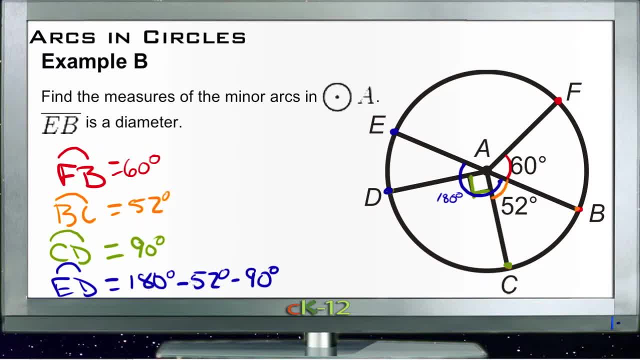 So 90 and 52 is 142, and 142 from 180 would be 38 degrees, like so. So this one here is 38 degrees. And then, finally, our last one is angle A and angle A right here. let's do that in pink. 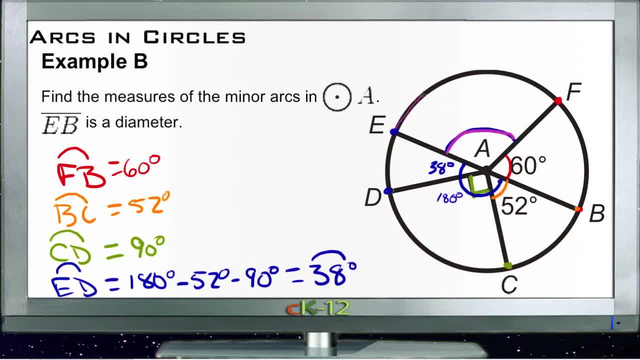 angle A, which is equivalent to arc EF. so we have EF. Arc EF is 180 degrees minus 60 degrees because it's the same diameter, but take away this section right here. So we have 180 minus 60 is 120.. 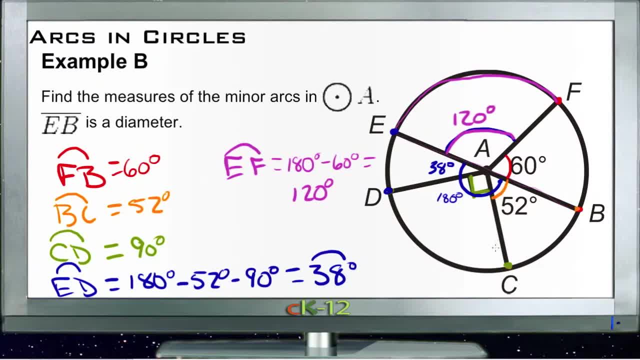 So this is 120 degrees right here. Make sense? Okay, so we have 120 degrees. What I'd like to do is see if we can keep this information right here, because we're going to need this one for the next one. 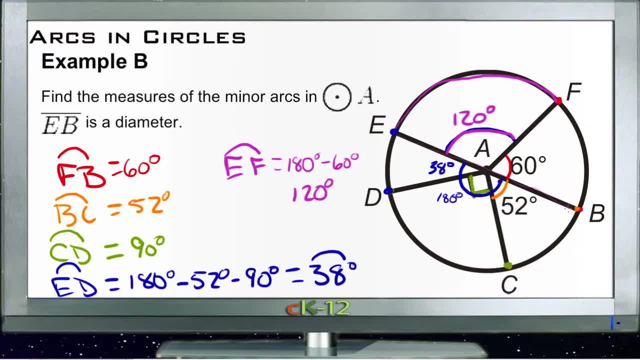 So let's pull this out. And our next one asks: Yeah, there we go, we can do that. We'll just pull. Let's just pull this right over here. We don't need this information right here. We'll get rid of that and then I'll have room for the other. 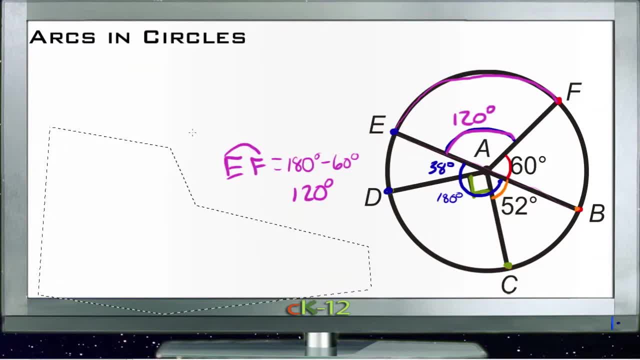 The next one wants to know what some of the combinations of those angles are. So if we get rid of this right here, then we'll have room for it. There we go, Okay, so C. example C asks us to find the measures of the indicated arcs in circle A. 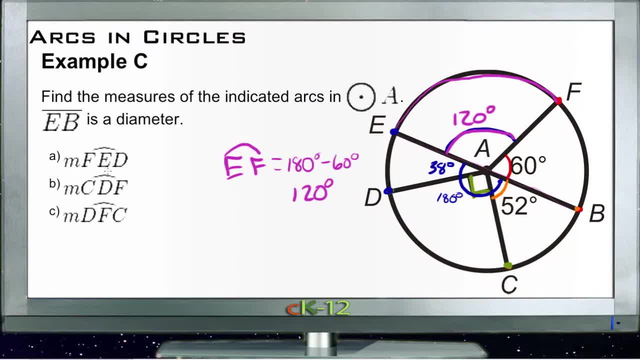 So the indicated arcs then are the measure of angle, FED, which is for angle A. Okay, So this is from here around to over here, so it's kind of an extension of minor arc, FE, right? So if we have the measure of FED, then it's going to be EF, which was 120 degrees. 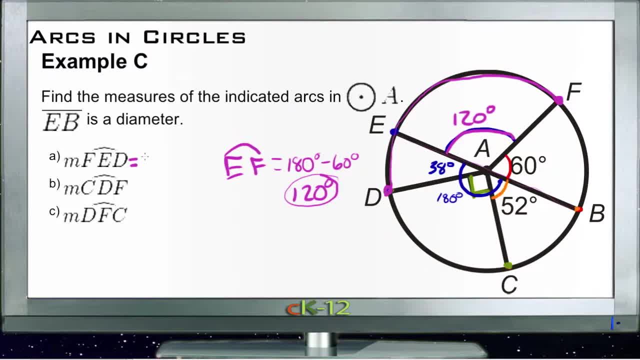 plus ED, which is 38 degrees. So we have 120 plus 38, or 158 degrees. So this arc clear around over here: 158, yep, okay. next one is CDF. let's get a different color. it's too red. 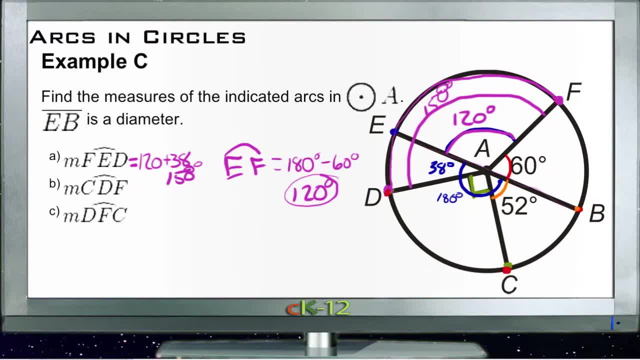 CDF would go from here to here to here, so that's definitely a major arc, right? That's most of the way around the circle, all the way around this outside section here. So that's going to be 360 degrees the whole circle, minus this 60 here and minus this 52 here. 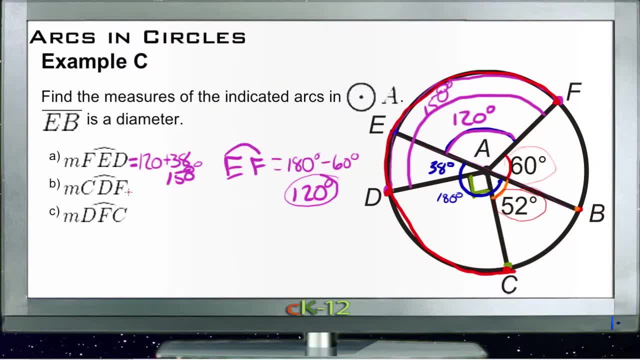 So 60 and 52 is 112.. So CDF, let's draw a line so we have a little more room. here is going to be 360 degrees minus 112 degrees, So we got 48, 248 degrees. So angle CDF or arc CDF, major arc CDF, 248 degrees, yep. 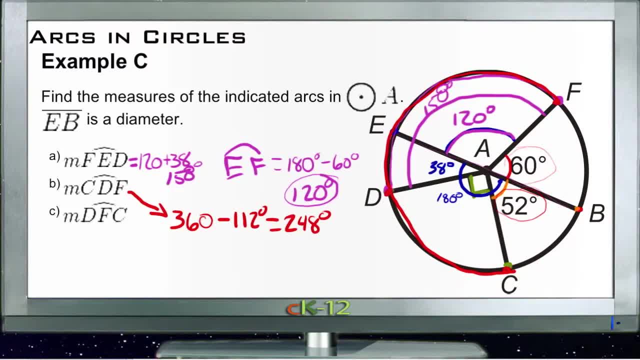 Then we have DFC. that's our final one, so it goes from: let's do that one in- oh, I don't know green, Yeah, So it's going to go from here, From here to here to here.